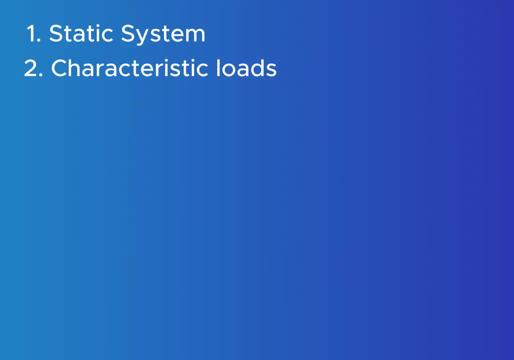 a static system for the timber beam. then we'll calculate all characteristic loads like dead load, snow load, wind load and live load. calculate all load combinations. choose a timber material. to find material properties then we have to assume the width and the height of the cross section to 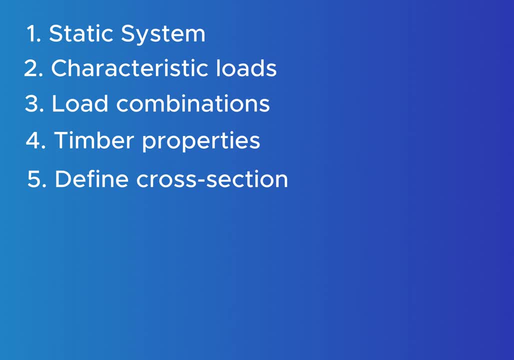 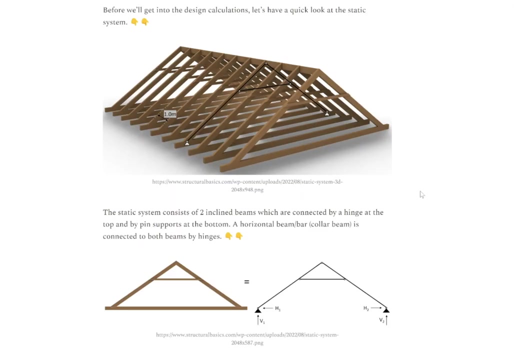 calculate the moment of inertia, verify the beam for bending for shear and then verify the beam for the instantaneous deflection criteria and for the final deflection criteria. Before we get into it, I want to invite you to my free newsletter. I send it out once a week. 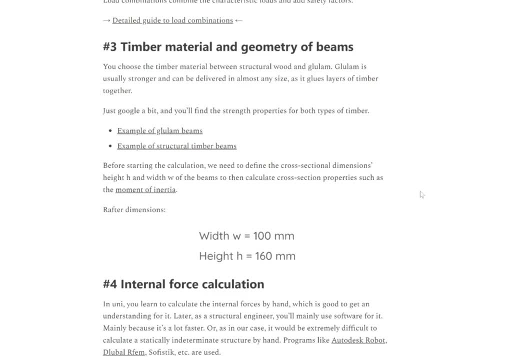 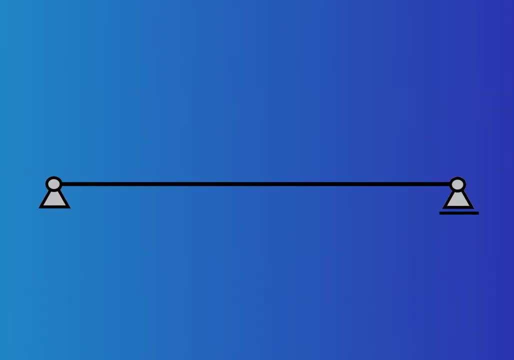 sharing structural design tips and tricks. You will find a link to it in the description below, So let's get straight into it. Most timber beams are simply supported beams, So we'll also use a simply supported beam as a static system, with one whip pin support and one roller support. To keep it in context with the 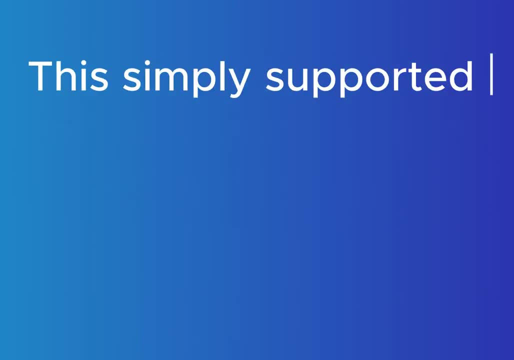 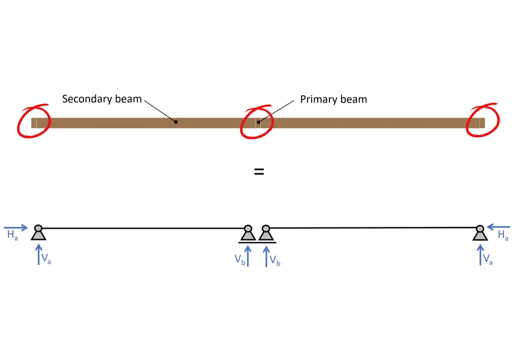 overall system of the flat roof. this simply supported beam can be a secondary beam in a flat roof. This gets a bit easier to understand when we visualize the secondary beams in a 2D section We can see that the secondary beams are supported by the primary beams. Now let's move on to the loads The beam needs to resist influences. 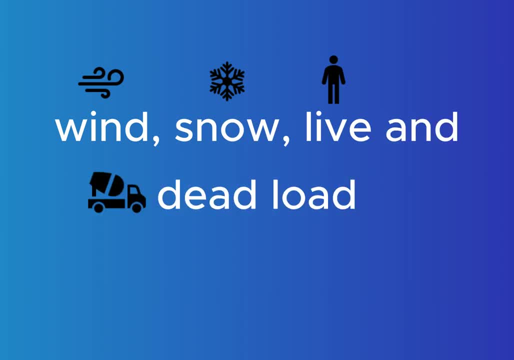 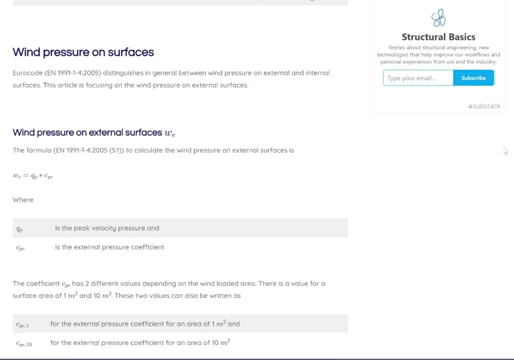 such as wind, snow, life and dead load. Now we can't show how to calculate these loads in this video, but we'll leave links to articles and videos that walk you through the calculations in the video description. For the design of the timber beam, we'll use a characteristic. 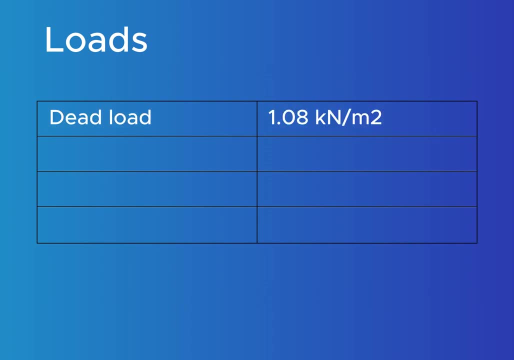 dead load of 1.08 kN per square meter, a characteristic value of the life load of 1 kN per square meter, a snow load of 1 kN per square meter and a characteristic wind load of minus 1.0 kN per square meter. Now, as a next step, we'll do load combinations. 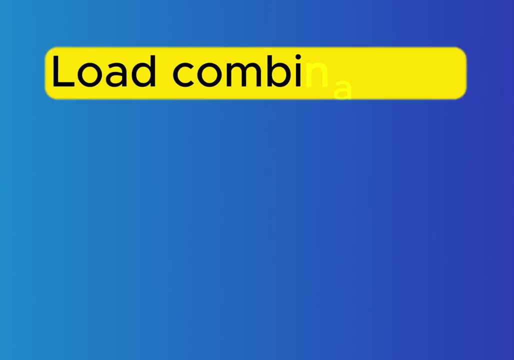 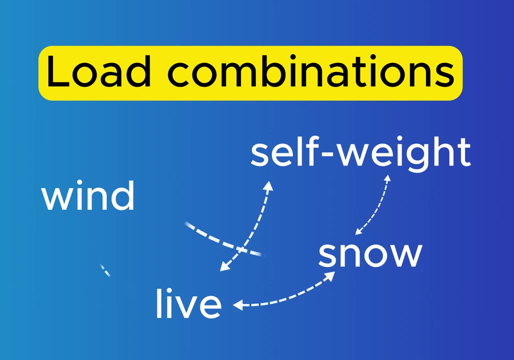 In short, as the name says, load combinations combine the characteristic loads, as we always design for the worst possible event that could happen Again. load combinations are a topic for another video, but you'll find a link to an article in the description below. 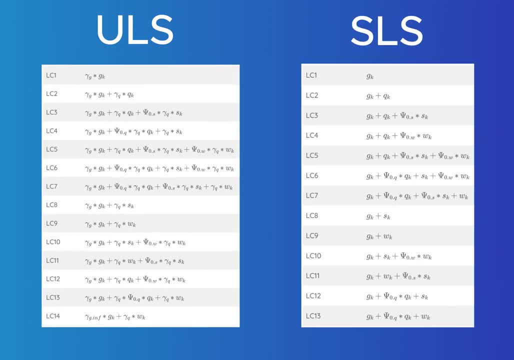 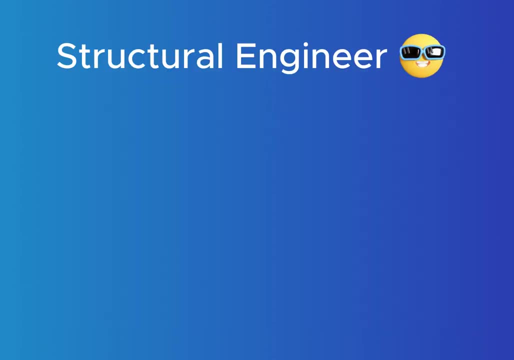 We define Ewell's and SLS load combinations and then use the load combinations with the highest value in our calculations. later on, The structural engineer needs to pick a timber material. Either structural wood or engineered wood such as glulam or laminated veneer lumber are used. 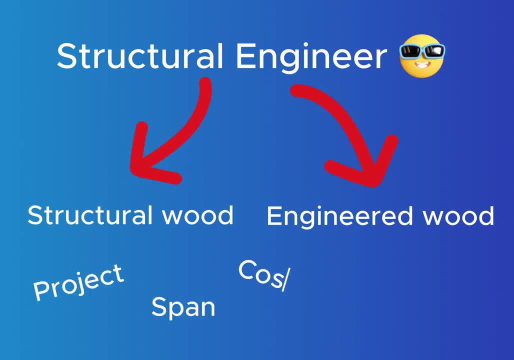 Which the designer picks depends on the project, span, cost and also personal taste. For our beam example, we're using a structural timber C24.. We can either use Eurocode or table from manufacturers to find these timber strength properties For this beam calculation. 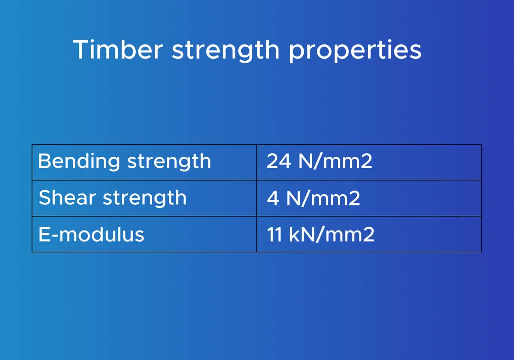 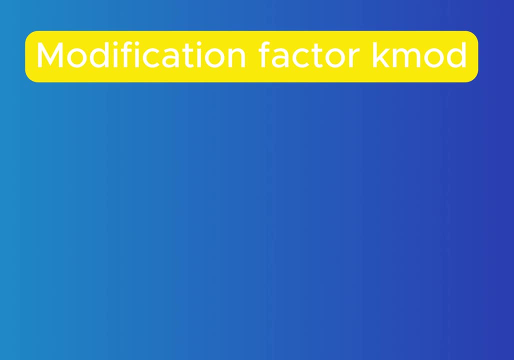 we need the bending and shear strength and the E-modulus. Now next up, the modification factor Kmod. This factor takes into account the effects of the moisture content and the load duration on the properties of the timber. This factor will be used to calculate the design resistance. 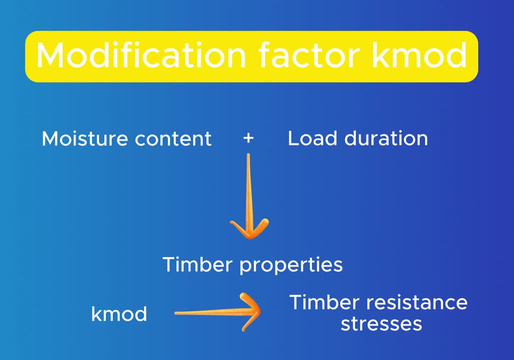 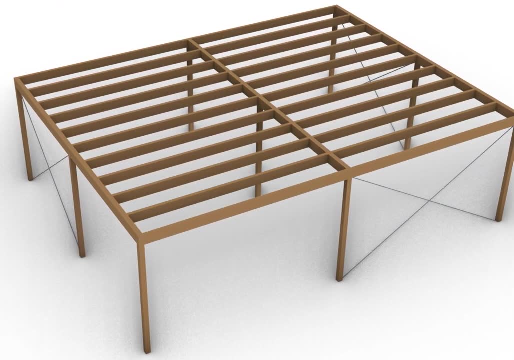 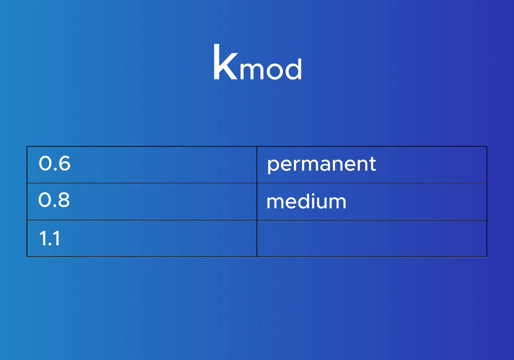 stresses in timber elements, Without going too much into detail for a flat roof of a residential house where the beams are not exposed to weather. we can define Kmod as 0.6 for permanent actions, 0.8 for medium-term actions and 1.1 for instantaneous actions. 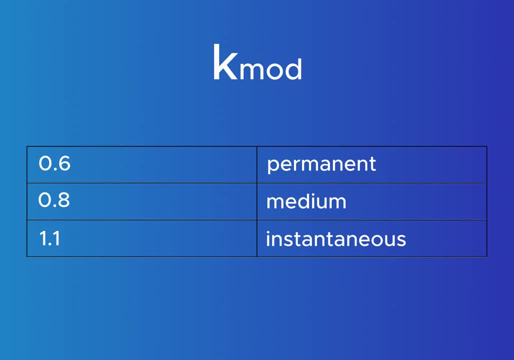 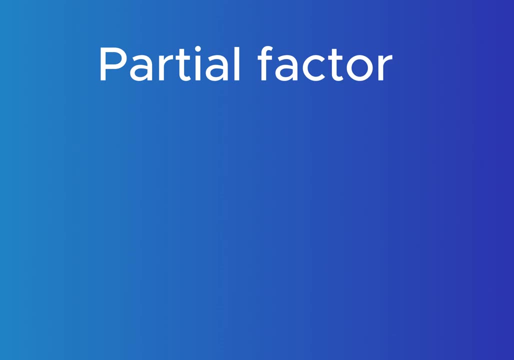 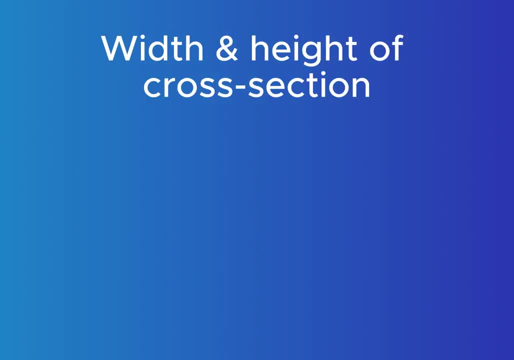 For this reason, we need to make sure that the beam is in the right position. For this reason, we need to define the width and height of the beam cross section to calculate the moment of inertia. This is based on the experience of the designer. We'll define the width as 80 millimeters and the 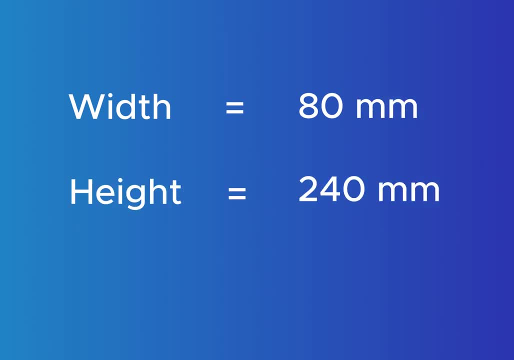 height as 240 millimeters. Once we know the height and width of the cross section, we can calculate the moment of inertia of the strong axis, which is needed to calculate the stress due to bending. We'll calculate the moment of inertia as 9.22 times. 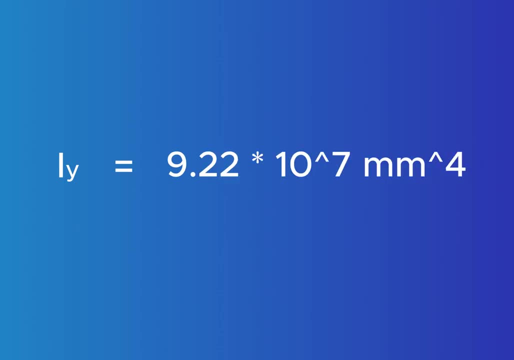 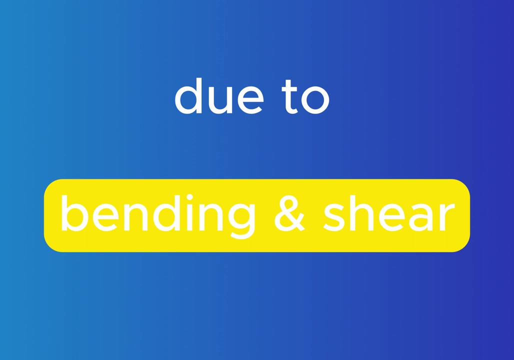 10. power of 7 millimeters. power of 4.. Now we're all set for the design of the beam In the ULS ultimate limit state design. we verify the stresses in the timber members due to bending and shear. Before we start calculating anything, we need to pick out the 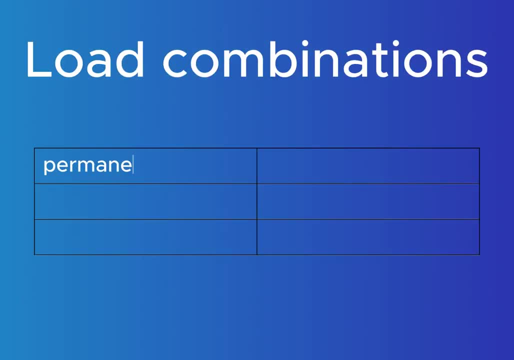 worst case load combinations for the permanent, medium term and instantaneous actions, meaning the highest values, because those actions lead to different resistance stresses Due to different K-mod values. Since we will design a beam in 2D, we need to transform the 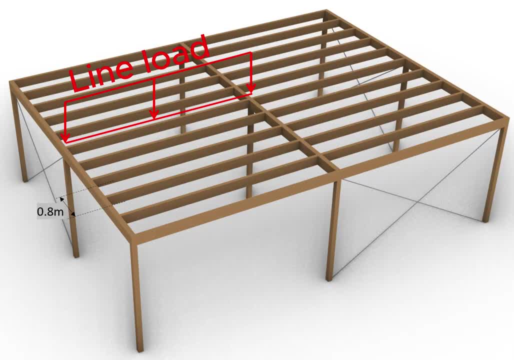 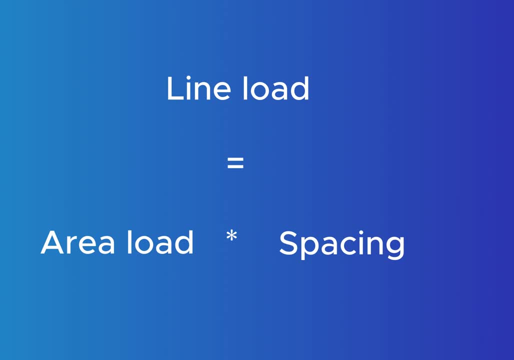 area loads into line loads. We do this by multiplication with the distance between the center lines of two beams. So for a beam with spacing of 0.8 meters we'll get a line load of 1.17 kilonewton per meter for load combination 1.. Those line loads can now be applied to our static system. 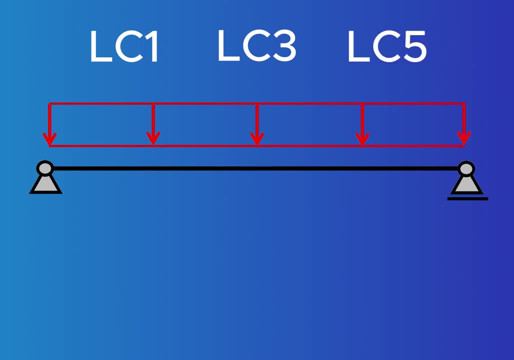 For the leading load combinations LC1,, LC3, and LC5, we can go ahead and calculate the most critical bending moment. The highest bending moment in a simply supported beam is found in the midspan and can be calculated with the most important formula in structural engineering: Q times L. 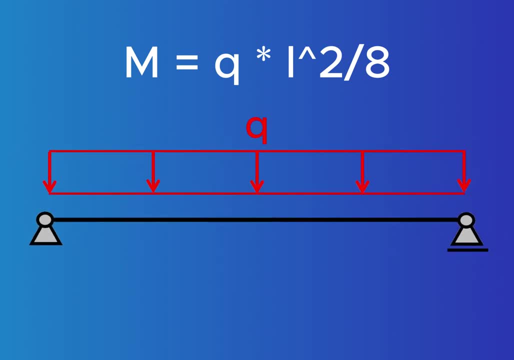 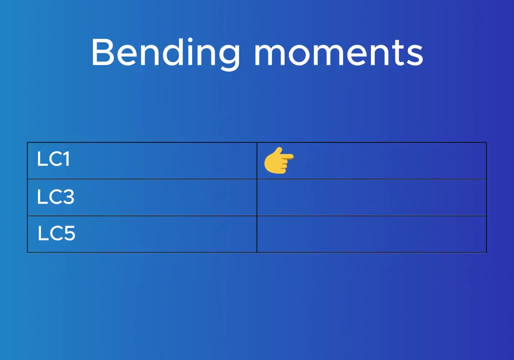 squared over 8, where Q is the applied load on the beam and L is the span. With this formula we can now calculate the bending moment for all three different load combinations. We calculate the stress in the most critical cross-section due to the moment as moment divided. 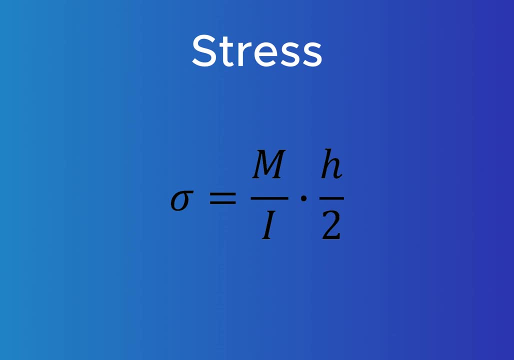 by moment of inertia times, half of the cross-section height. Again, we do that for all three load combinations. In the last step, before we can actually check whether or not the cross-section can resist the load, we have to calculate the resistance stresses of the timber materials. 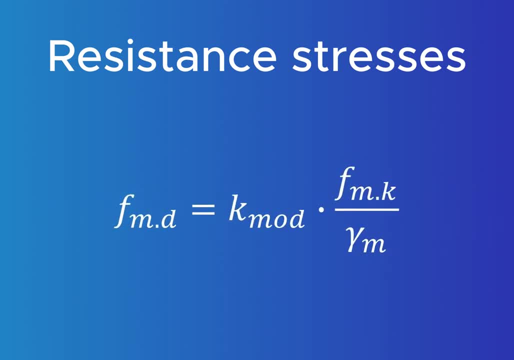 We do that by calculating K-mod times, the bending resistance of the timber material divided by the partial safety factor. Because we have three different K-mod values, we also get three different bending resistances. Okay, now let's check if the utilization is less than one by dividing the resistance stresses. 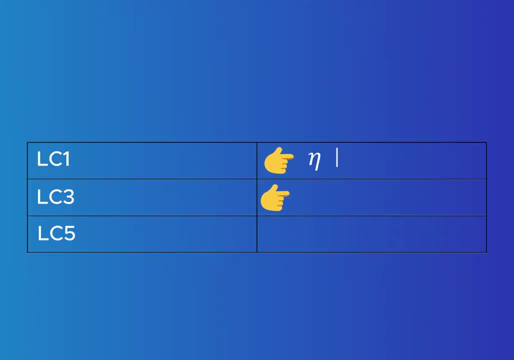 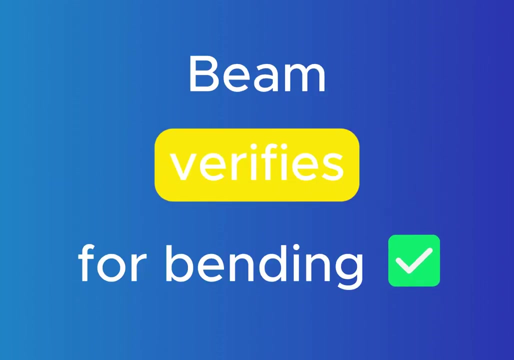 through the design stress. As we can see, the highest utilization is 0.88, which is less than one. This means that the beam verifies for bending. That's great, and we can now move on to shear. First we'll calculate the shear. 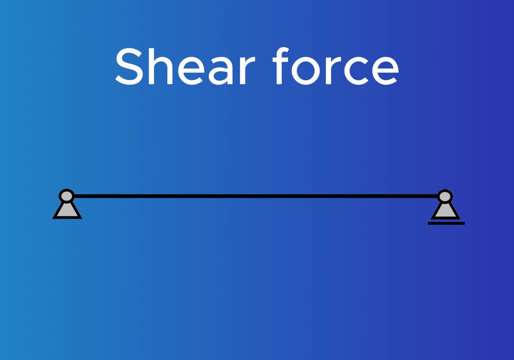 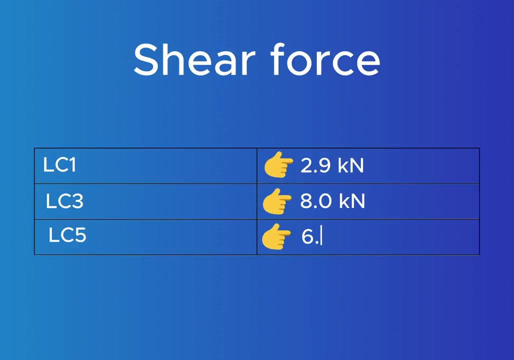 The highest shear force in a simply supported beam is found near the two supports and is calculated as Q times L over 2, where again Q is the applied load on the beam and L is the span. We do that for load combinations LC1,, LC3, and LC5.. With the shear forces we can now calculate. 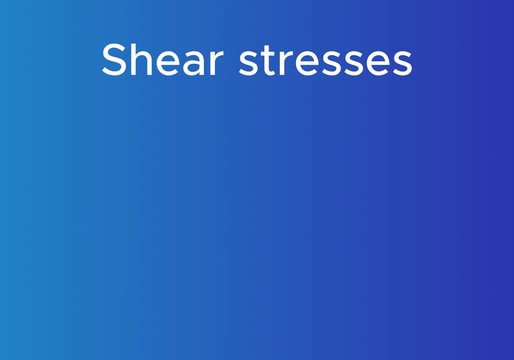 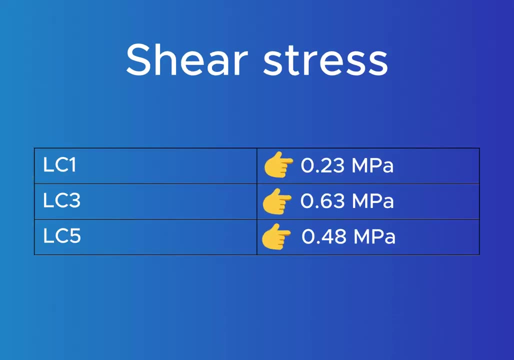 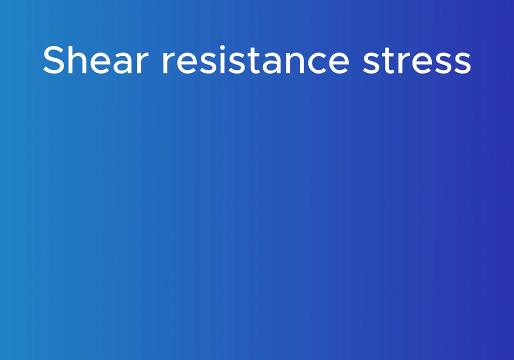 shear stresses in the most critical cross-section as 3 over 2 times shear force over cross-section width times cross-section height. The last step before we can check whether the cross-section can resist the loads is calculating the shear resistance stresses of the timber material as K-mod times. 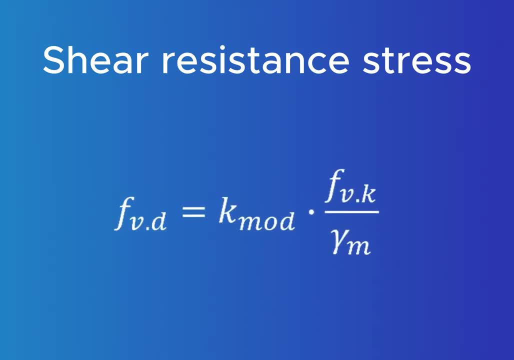 shear resistance, stress over partial safety factor. And finally we can calculate the utilization of the cross-section with design shear stress over design shear resistance. We can see again that load combination three leads to the biggest utilization, but it's far from one. The load combination 3 leads to the biggest utilization, But it's far from one. 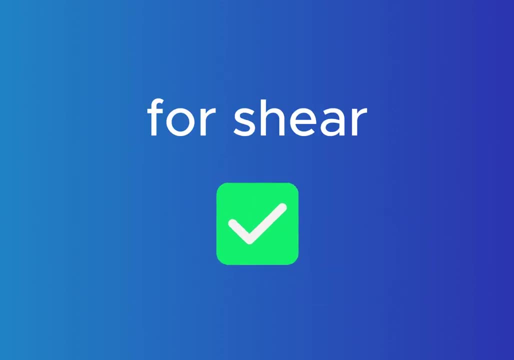 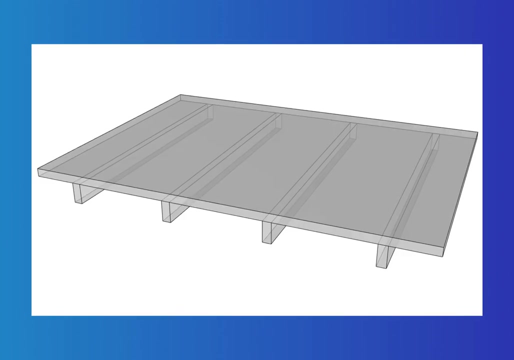 So the beam is also verified for shear. Now, moving on to the SLS design. In the SLS design of a beam, we verify that the deflection does not exceed values defined either in Eurocode or values from the client. And in case you use timber beams in ceiling systems, you should also verify vibrations. 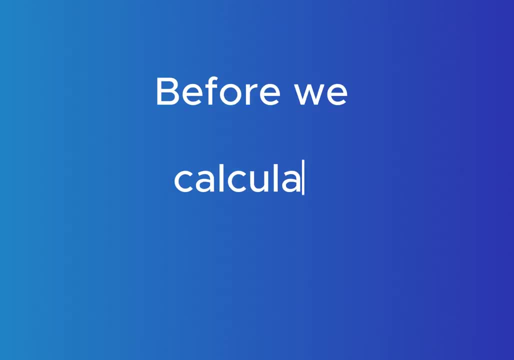 But as we are designing a roof, we don't need that step. Before we start calculating anything, we need to define a few variables. So table 7.2 of Eurocode 5 recommends ranges for the instantaneous and the final deflection, which should not be exceeded for a simply supported beam. 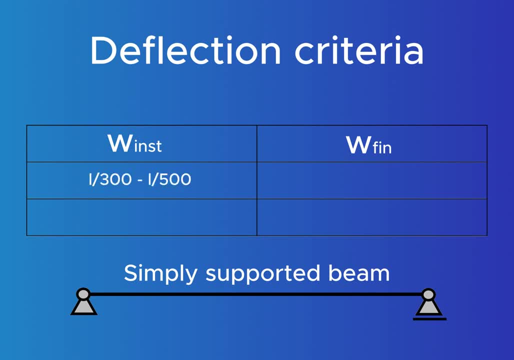 The instantaneous deflection should not exceed L over 300 to L over 500.. For a 5 meter long beam, this is a range of 16.7 millimeter to 10 millimeters. The final deflection should not exceed L over 150 to L over 300. 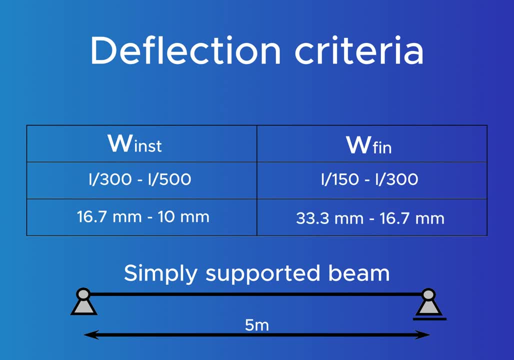 This results in a range of 33.3 millimeters. This results in a range of 33.3 millimeters to 16.7 millimeters. Alright, now let's have a look at how to calculate the deformation. The instantaneous deformation of our beam is calculated with the load of the characteristic load combination. 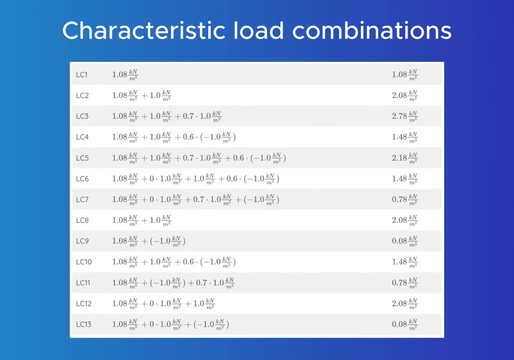 Looking at all load combinations, we can see that LC3 leads to the biggest load, where the live load is the leading and the snow load the accompanying variable action. Now we need to transform this area load into a line load by multiplying it with the spacing of the beams of 0.8 mm. 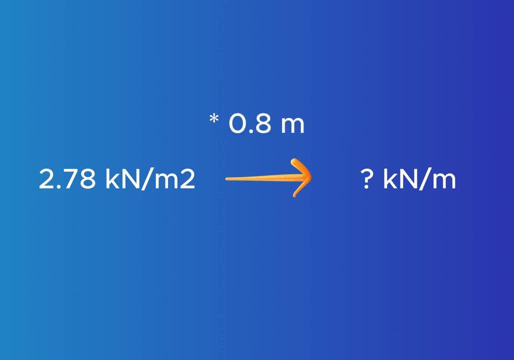 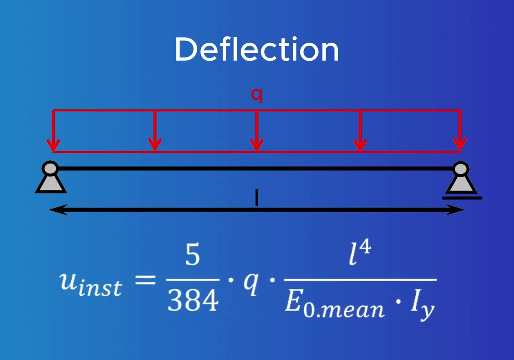 Which leads us to a line load of 2.2 to kN per meter. The deflection of simply supported beams exposed to line loads is calculated as 5 over 384 times the load times L to the power of 4 divided by E-modulus times. moment of inertia. 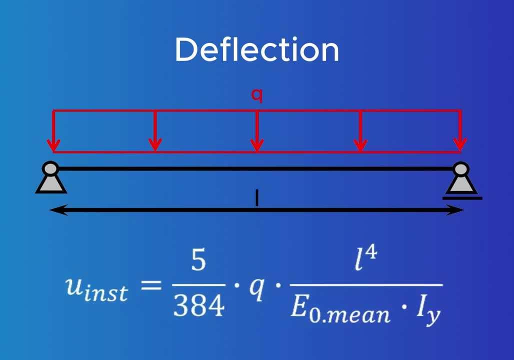 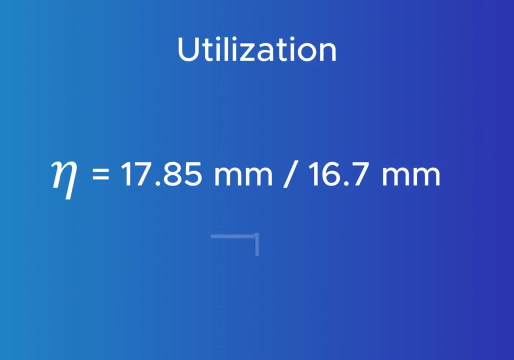 This leads us to instantaneous deflection of 17.85 millimeters. Now, when we calculate the utilization, we find out that it's greater than 1.. This means that the beam deflection is greater than 1.. This means that the beam deflection is greater than 1.. 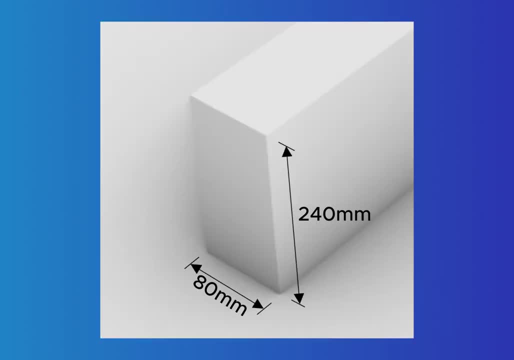 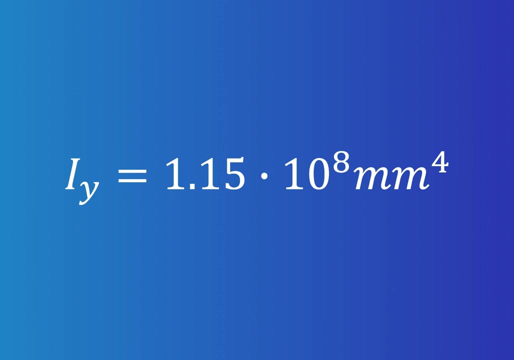 The deflection does not fulfill the deflection criteria and we have to change the cross-sectional parameters. Now we increase the width from 80 mm to 100 mm and recalculate the moment of inertia as 1.15 x 10 to the power of 8 mm, to the power of 4.. 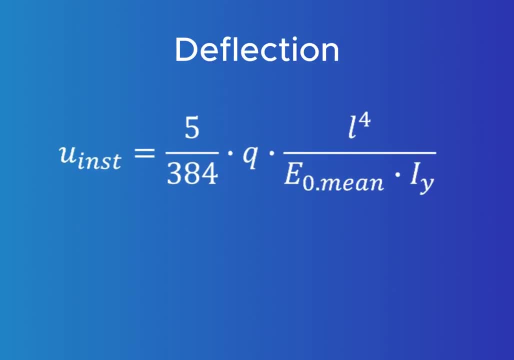 Now we run the deflection calculation again with updated dimensions and get an instantaneous deflection of 14.28 mm. Now we run the deflection calculation again with updated dimensions and get an instantaneous deflection of 14.28 mm. Also, the utilization is less than 1 now. 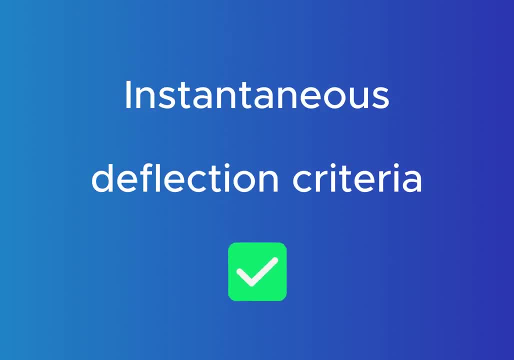 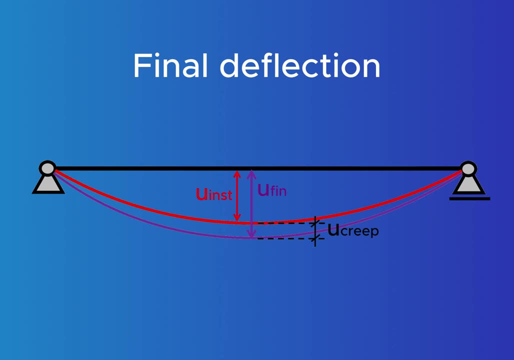 Now, finally, the instantaneous deflection criteria is verified. The final deflection of our beam can be calculated by adding the creep deformation to the instantaneous deflection. Therefore, we will look at how to calculate the creep deflection of float combination 3.. We calculate the creep deflection separately for dead live and snow load, as we are adding. 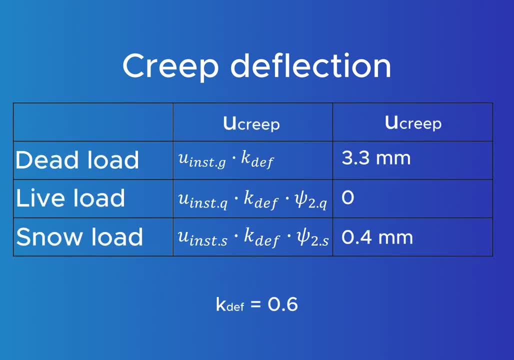 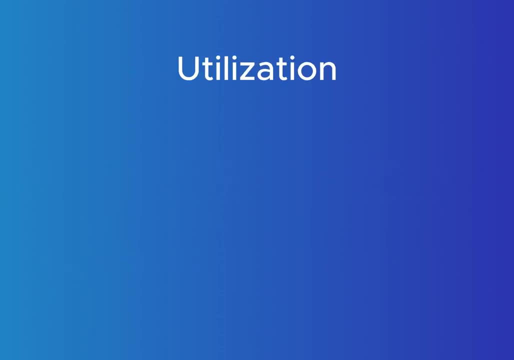 factors to live and snow load. Finally, we calculate the final deformation by adding the creep deformations to the instantaneous deformation. This leads to a utilization of 0.54.. And therefore the final deflection criteria is verified and the whole beam is basically verified for the dimensions of 100 mm in width and 240 mm in height. 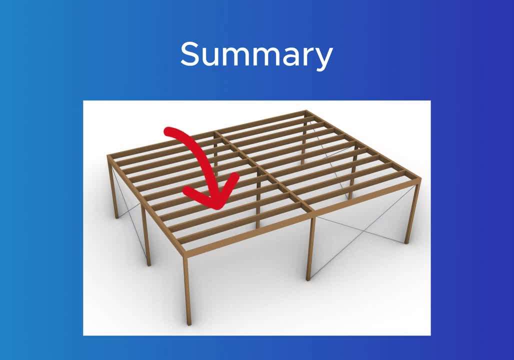 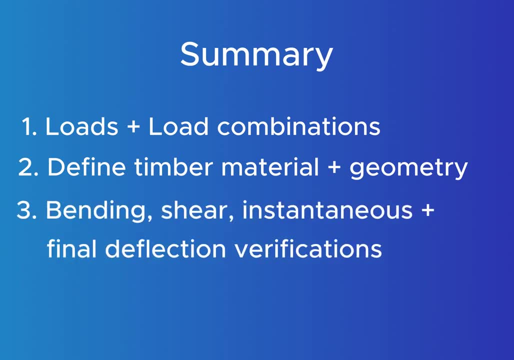 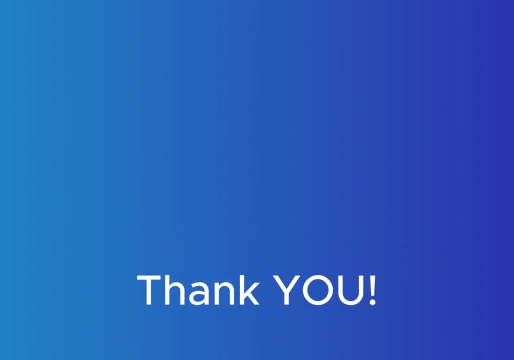 To summarize: to design a timber beam, we have to first calculate the loads and load combinations, define the timber material and beam geometry, Verify the beam for bending shear, instantaneous deflection and finally the final deflection. Thanks for watching. If you enjoyed this video, please give us a like. 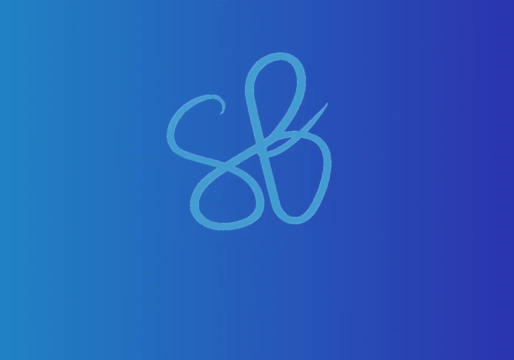 You can also find other structural engineering guides on our homepage, structuralbasicscom. Until next time.